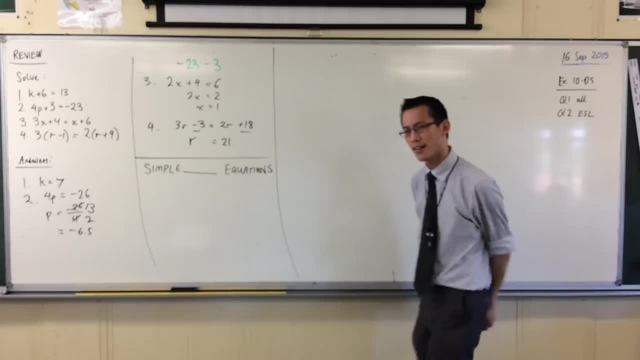 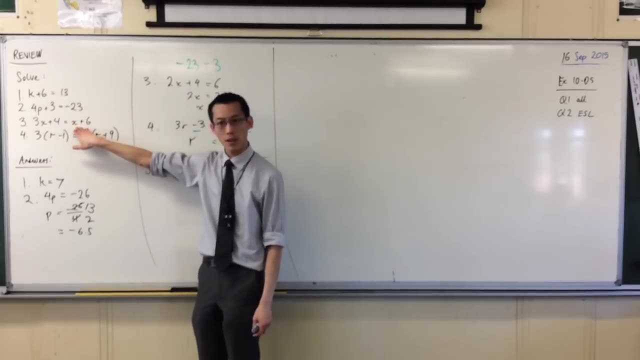 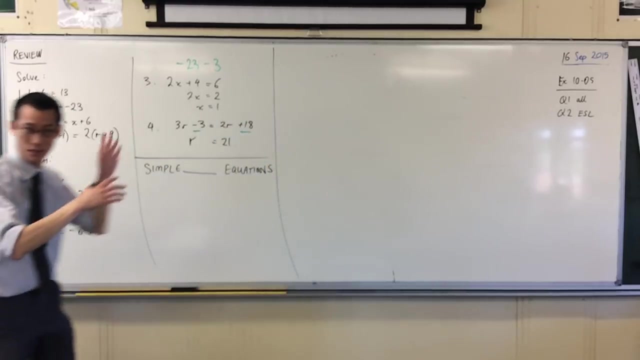 Hmm, Think carefully How much- Yeah, I don't know. Letters are here. I have some here as well. I guess a way I could say this is: In fact, you may like to go back to your original question and add this on, so you can have some language. 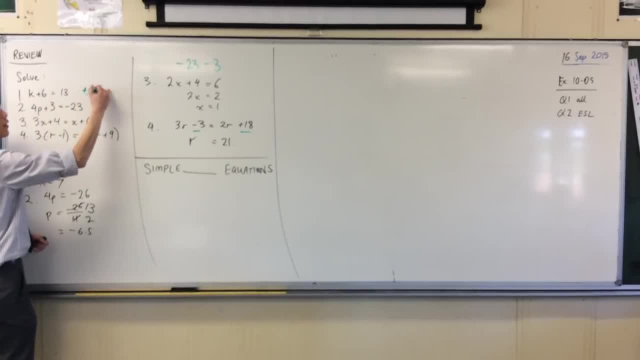 for describing what's happening Here. we're adding and we're subtracting numbers, right? That's what plus 6 is. We're Multiplying and dividing by numbers, right? Do you see that, Like there's 4 at the front? 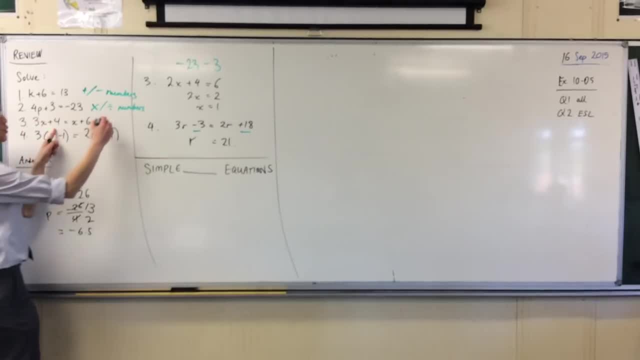 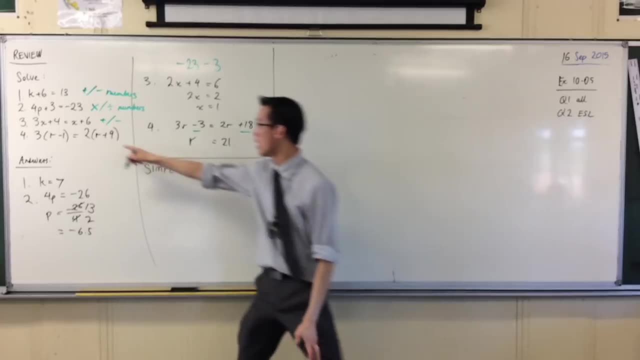 which is multiplication. And then, for this one, what we're doing is we're adding or subtracting- not numbers, but pronumerals, right, Like more Xs or more Rs or Ks or whatever. okay, So I'm going to write pronumerals here, All right, Now I just want you to carefully look. 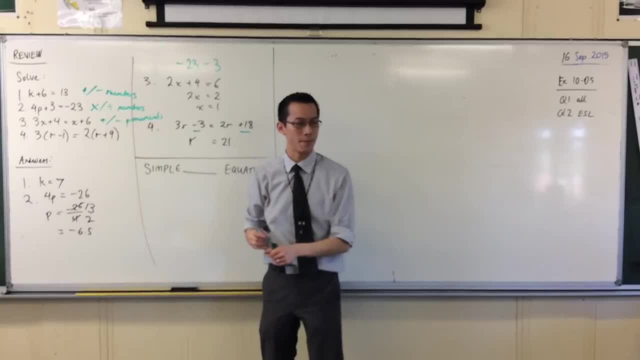 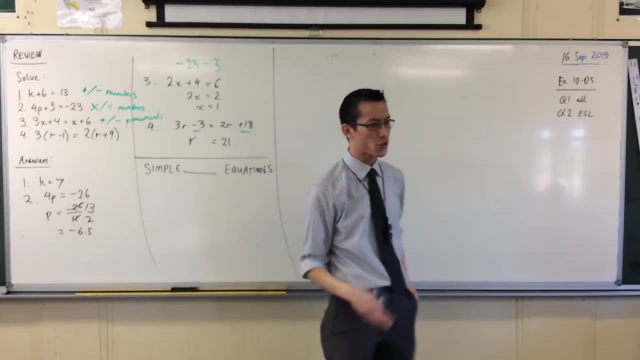 at what we've just established right. I know I've got brackets there, but I'm not going to worry about him for now. You can add subtract numbers. You can multiply and divide numbers. You can add subtract pronumerals, If you were trying. 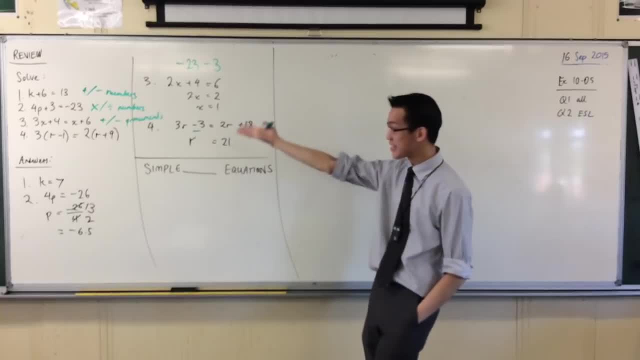 to complete the pattern. what's the next step? What's missing from this list? What looks like it should be the next thing? Yeah, Nathan Times, and divide, Multiplying and dividing, but not by numbers, by pronumerals. okay, What would happen to? 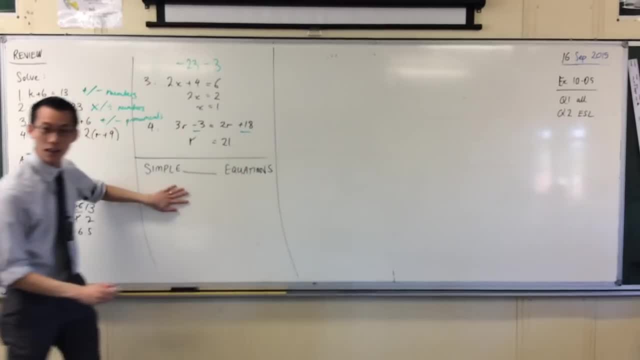 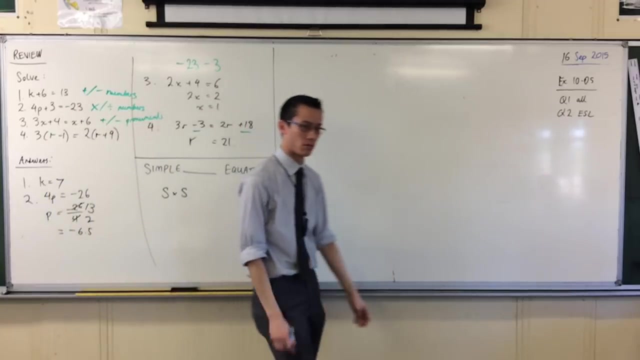 equations. right, An equation if, for instance- and this is what you can write under your new heading- If I had, let's go with the letter like, say, let's go with the letter S If I had S and instead of adding or subtracting a pronumeral, what if I multiplied by a pronumeral? 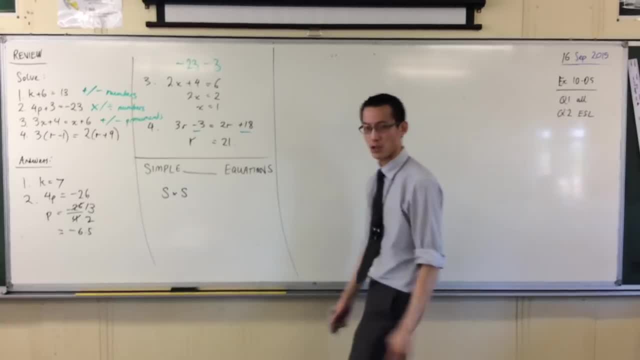 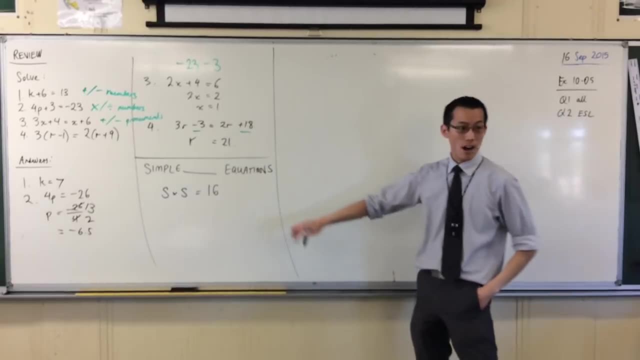 okay, Now I want to make an equation. I'm trying to deal with equations here, right? So, just as an example, I want to pick out the number 16, because I like the number 16,, sweet 16,. okay, Now, this is our example. So I'll just write example at the front: We 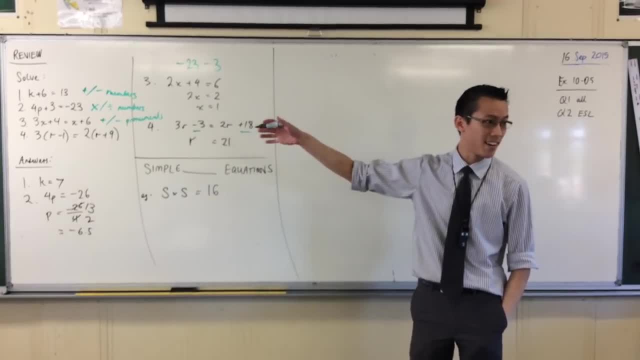 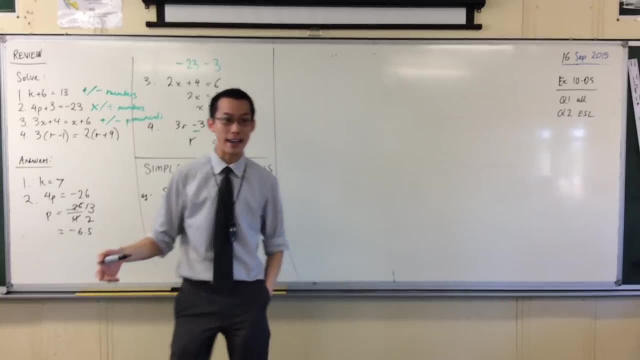 have some language. We already developed some language earlier this year. to write this in a more concise form: Do you remember what language we used? Start it with an I Index form right. Very good, So S times S I'm multiplying S by itself. 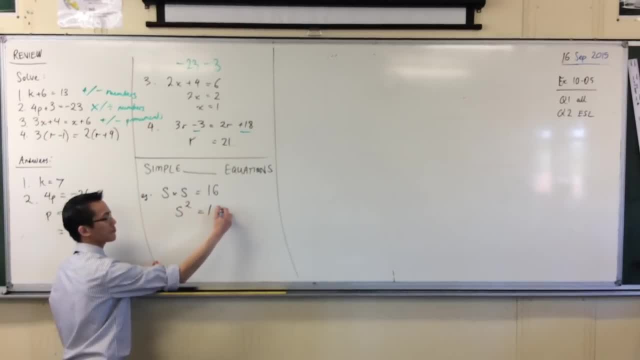 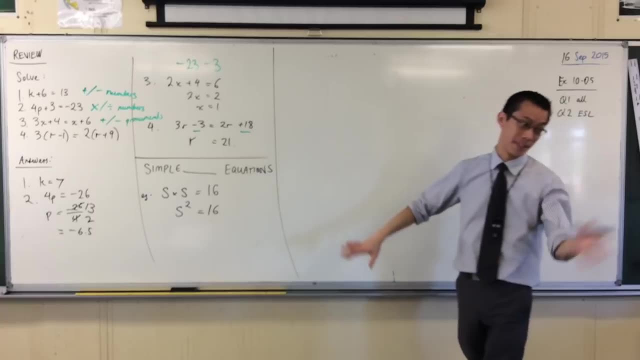 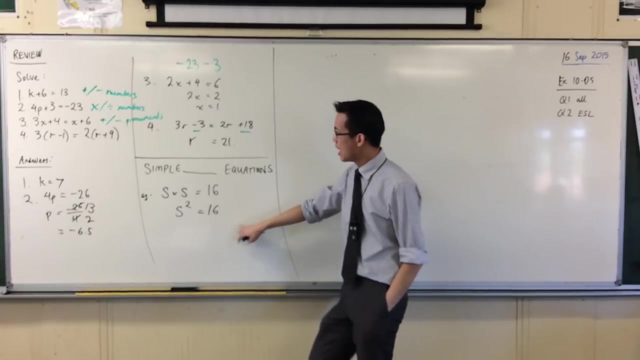 twice. so I write S squared. okay, Right now. Adam, yes, Okay, so we'll get to the names in a second. Let's just worry about what it is. but yes, okay, We have a look at this equation, right? This is a bit strange because you know how. 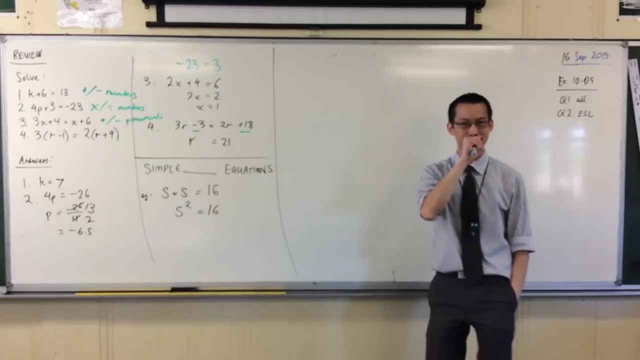 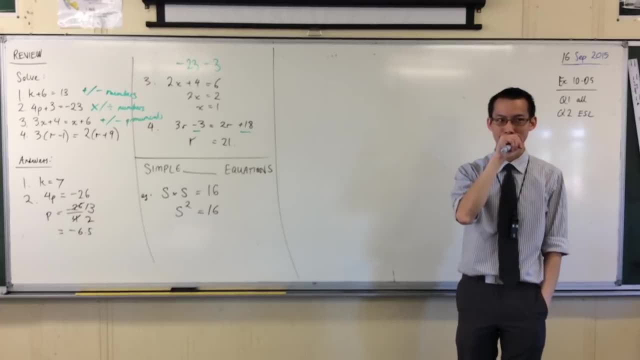 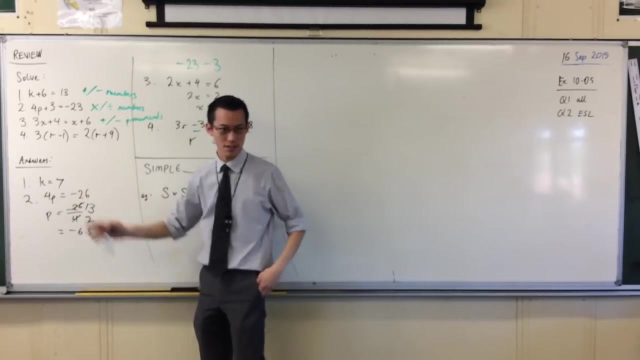 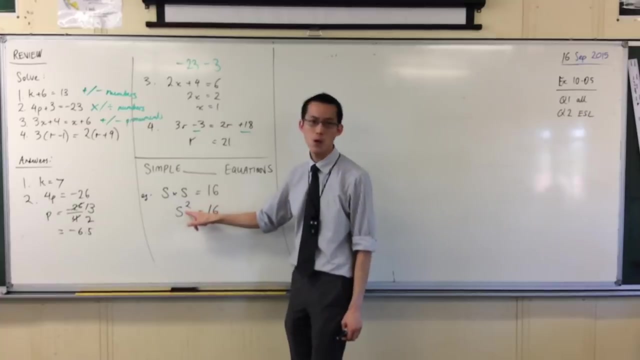 before we said. Before we said the goal was to get the pronumeral by itself. how to do this? The pronumeral kind of looks like it's already by itself. right, Almost right. There's just this two hanging around. So we're going to do this thing to solve it. okay, Now, before I jump, 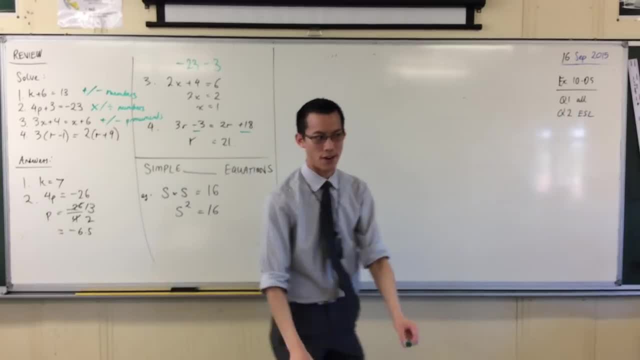 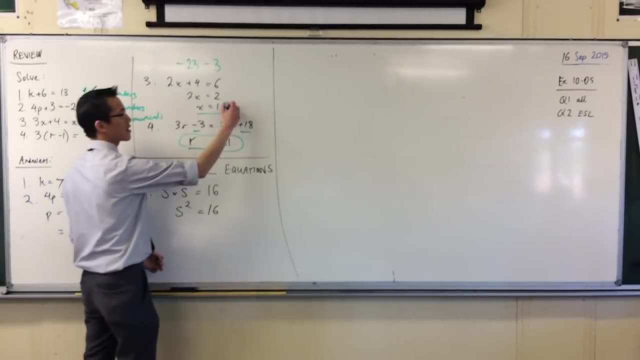 to suggestions. I just want you to remember- we've been saying it over and over again. I hope you're a bit sick of it really- The reason why R equals 21 is a solution and the reason why R equals 1 is a solution. 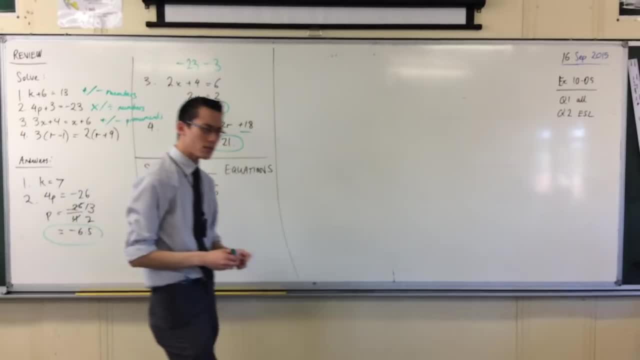 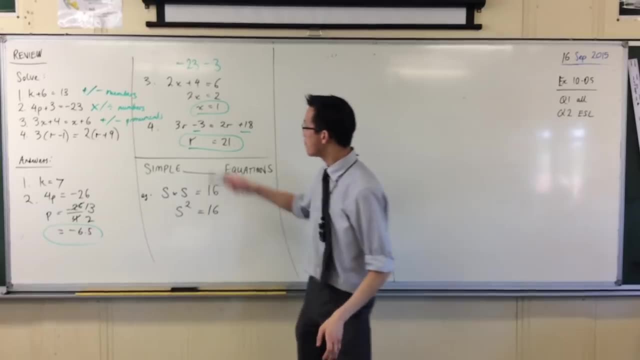 and P equals minus 6 and a half, and on and on and on. The reason why they are solutions is because you can put those numbers where. Where can I put them? Yeah, back into what I started with. right, I could put R equals 21 in here, and it should. 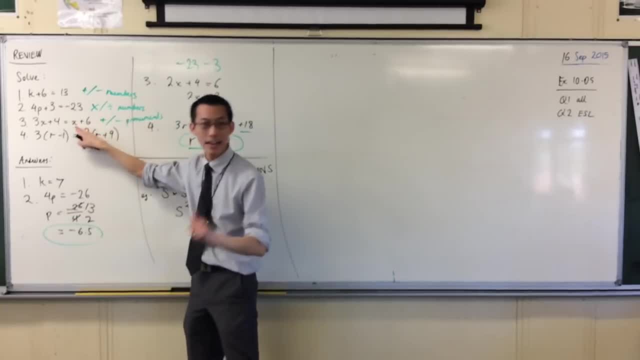 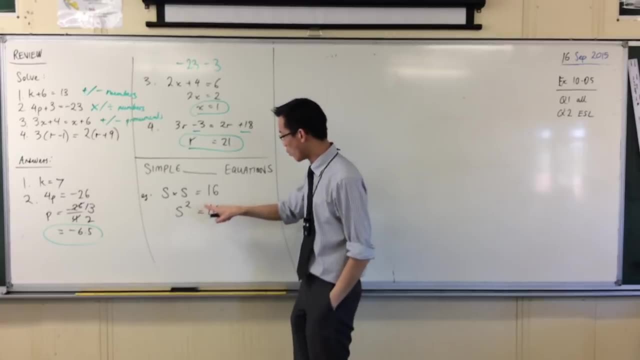 work. I could put X equals 1 in here and it should work. So I want to think of what number, What number can I put in here for S that would work with this? And it's not what you think of, right, Daniel? what would you put in there? 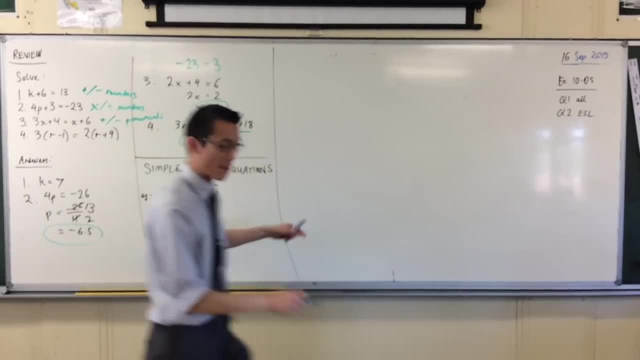 I would put in 4.. I would put in 4.. In fact, underneath here, let's just write that down right? If you've got another color, that'd be helpful. 4 squared does equal 16.. I could. 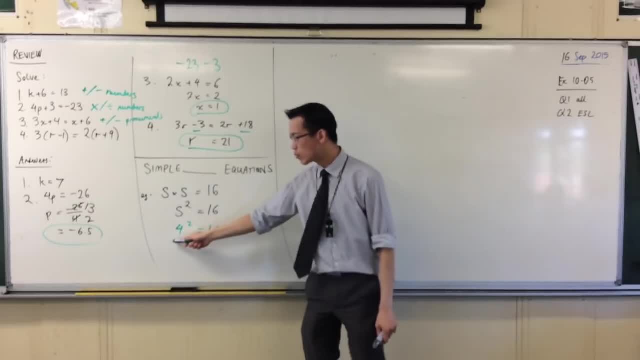 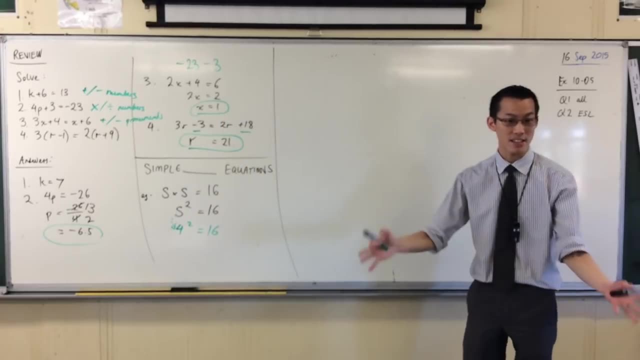 pop it in and it works. So S equals 4, see that S equals 4 is a solution. okay, That's great. There's something a bit sneaky going on here, right, Unlike every other question we've been. 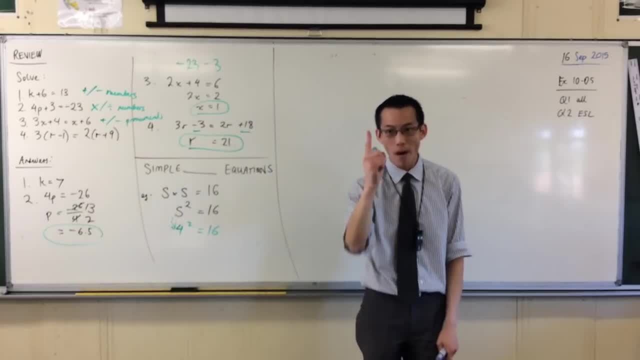 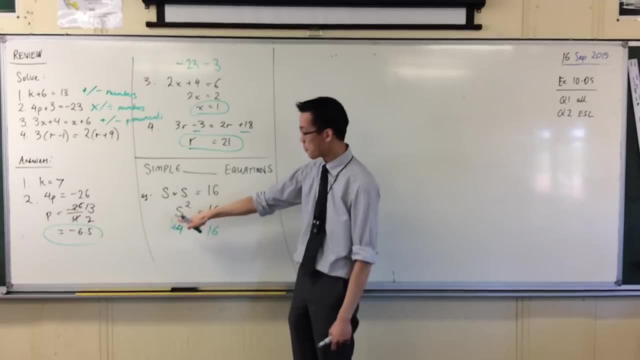 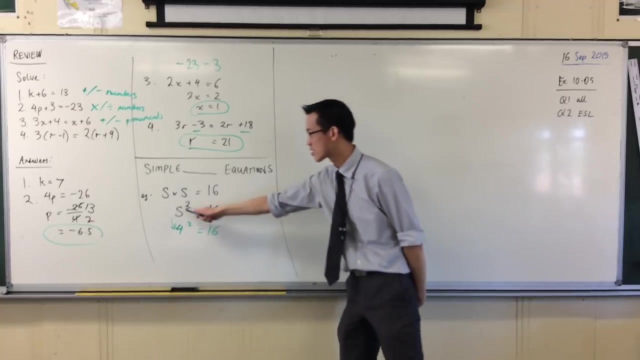 doing where, when you solve it, there's a solution, one solution. There's actually another number that I can put in. I can substitute it, I can swap it out for S, and it will still work. It will still be a solution. Can anyone think of another number that I can square? 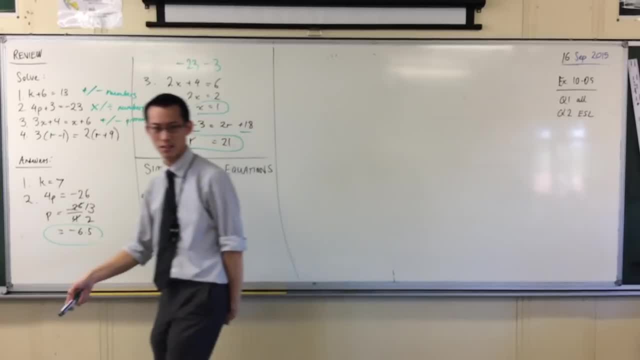 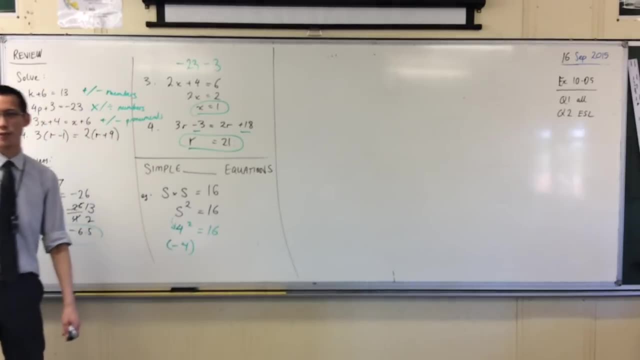 and it'll give me 16? Will, Minus 4.. If I take negative 4, right. And if I square it right, When you square a negative number, let's just write this out: that's minus 4 times minus 4, right. What happens to those? 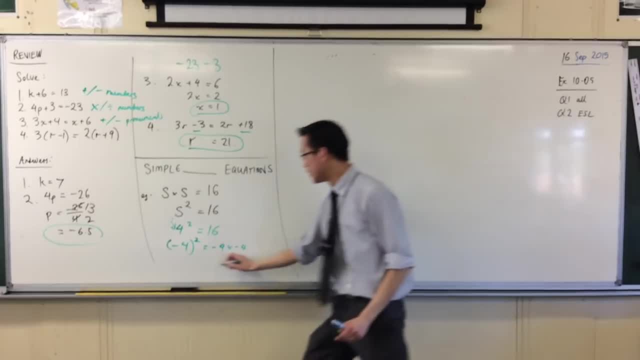 negatives, They become positive, They cancel each other out, leaving you with 16, right. So since minus 4 squared also equals 16, it also works for this equation, right. S can be both of these. It can be two values, It can be one or the other, right. So I've 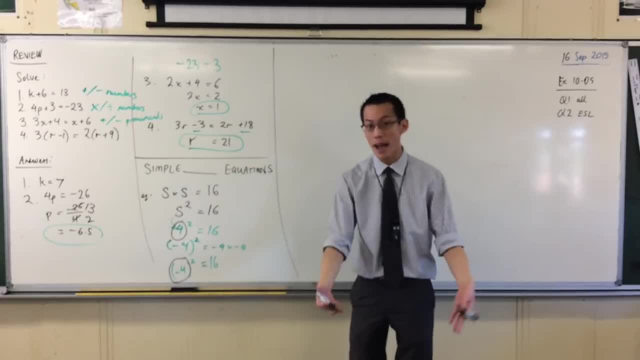 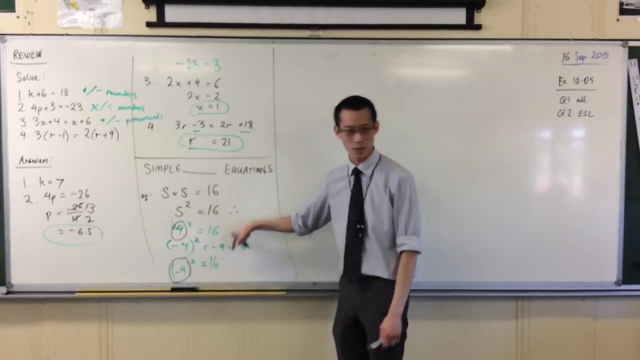 got this guy here and this guy here. So the way I write this being that one is positive 4 and one is minus 4, I would say I've run out of space. I would usually put this underneath, And you guys can put it underneath. I would write S equals. we have a symbol for this. 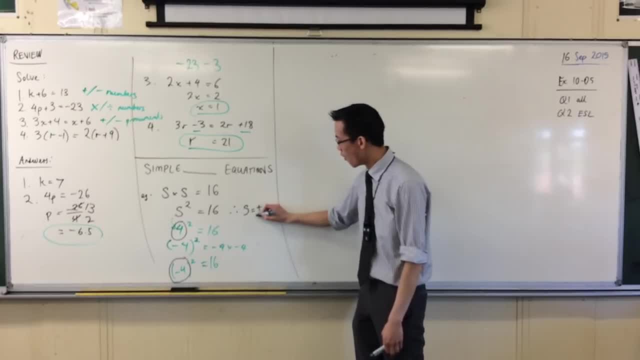 because it happens so often: plus or minus 4, okay, You might have seen this before. actually, I literally read this as: S equals plus or minus 4.. It's kind of like a shorthand to say two numbers at the same time but cramming it into the one spot, okay. 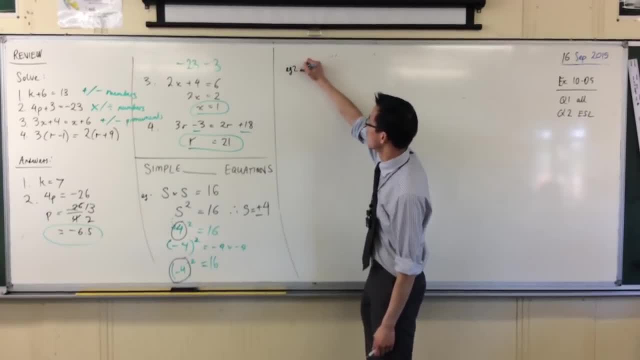 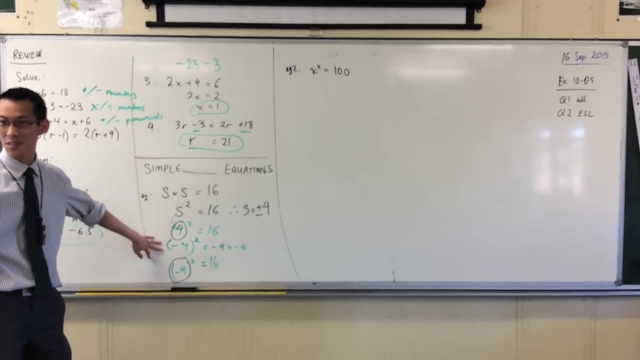 So, for instance, if I gave you another one, if I said: this is example 2, how about X? squared? oh, how about? okay, Now, every time you see this square thing happening, because of what you notice down here, there's not just one solution. 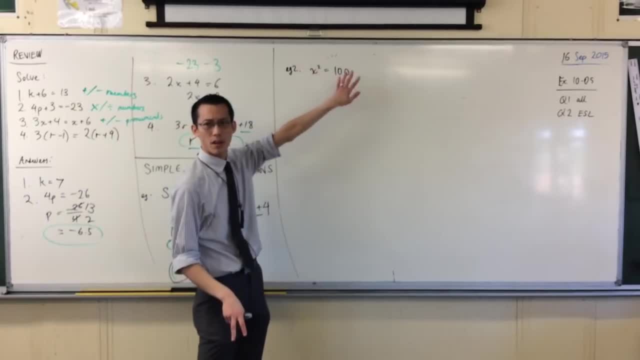 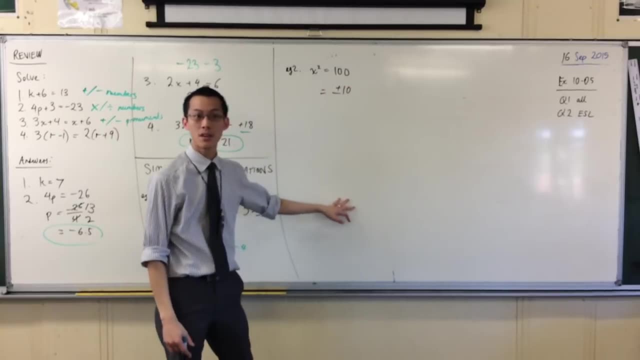 There are two. What's the root of 100?? What number is it? Yeah, It's 10.. It's going to be. the solution to this is plus or minus 10.. And the root of 100, put either of those. 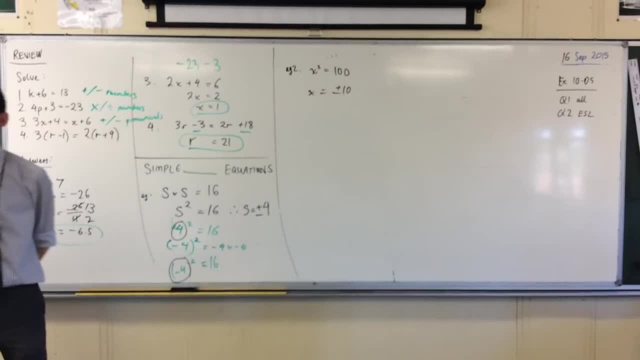 numbers in here and it works. Yes, Is it true that there are no square roots for negative numbers? We'll get onto that, We will. It takes a lot of time to get to that, but let's just contemplate for a second. Let's do example 3, and it's worth writing this down for everyone, because 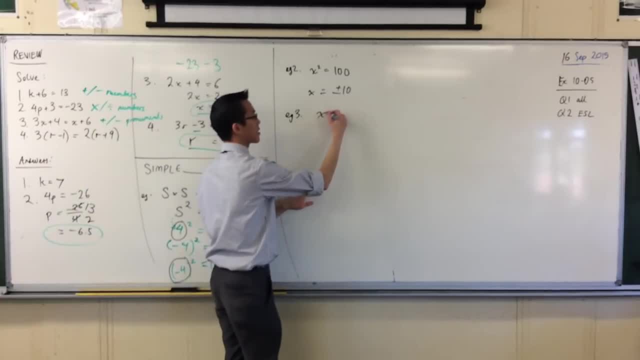 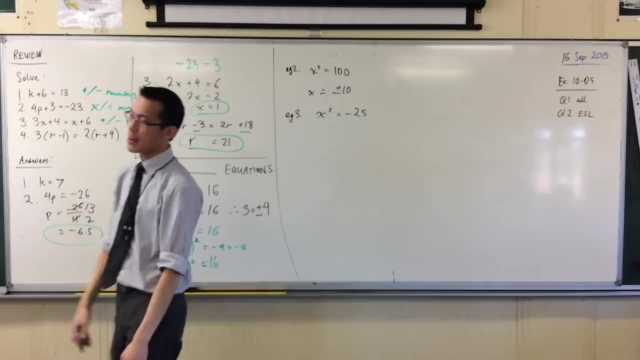 it's a question you will get asked If I said: well, I don't know, minus 25,. okay, Minus 25.. Now, if I start thinking about all the numbers that I know about, right, Can you give me some examples of what families? 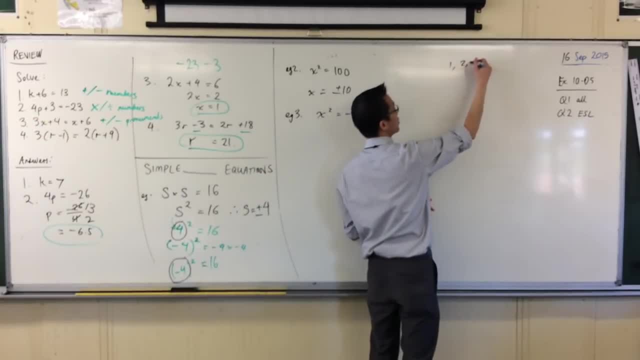 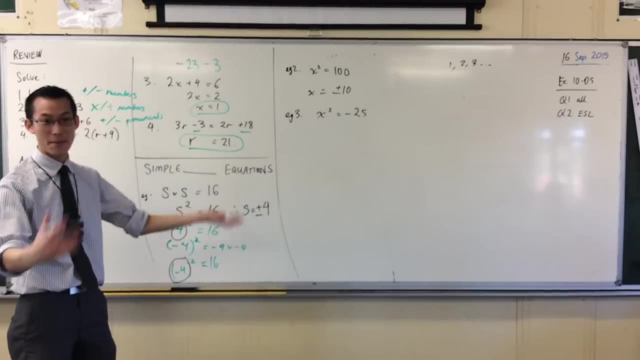 of numbers do I know about? I'll give you an example. first, One, two, three. What would you call those numbers? They're the numbers that are. they're a couple of names. The fancy name is the natural numbers. These numbers come from counting like one, two, three. 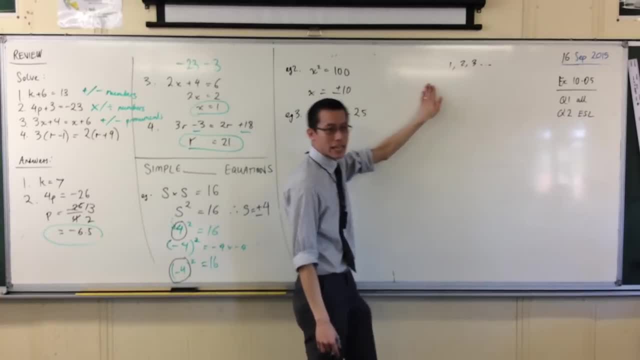 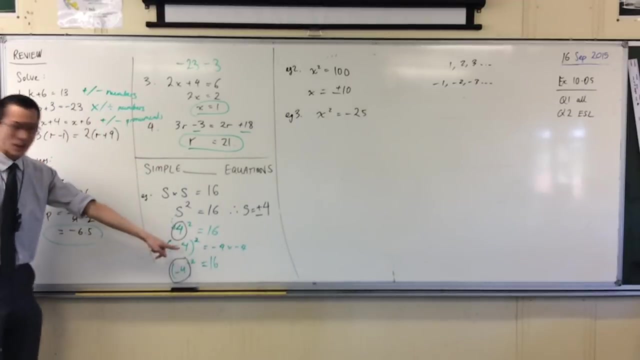 You call them the counting numbers, right? Can you take any one of these numbers and square it to get minus 25?? Okay, Now, if I try, for example, not a counting number but an integer, they've got negatives right. I run into a problem because this will happen. 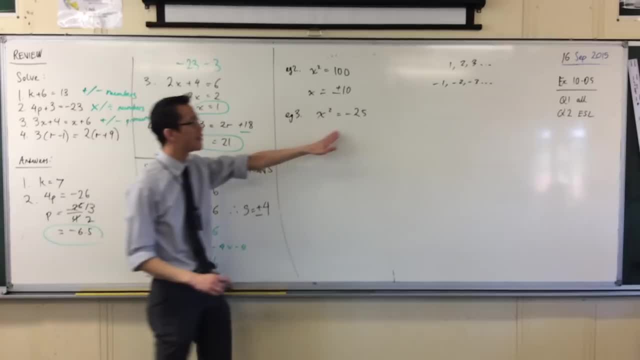 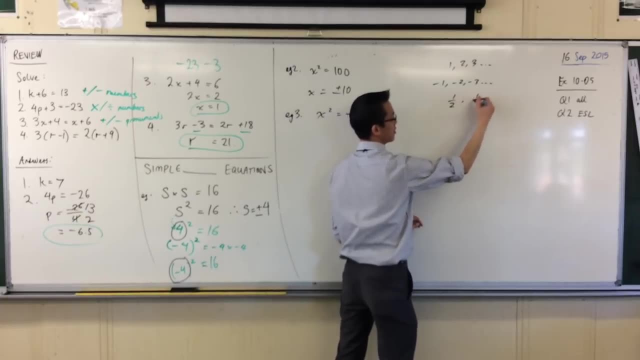 right, The negatives will cancel each other out. I will never get minus 25.. Even if I try like weird numbers, like, say, the rational numbers, the four, the four, the four, the fractions, like that. You could even try weirder numbers, like the square roots, like 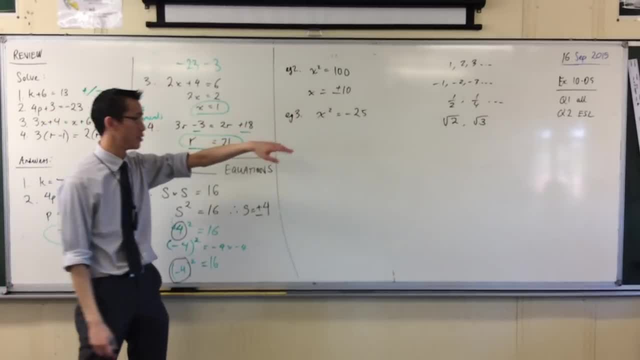 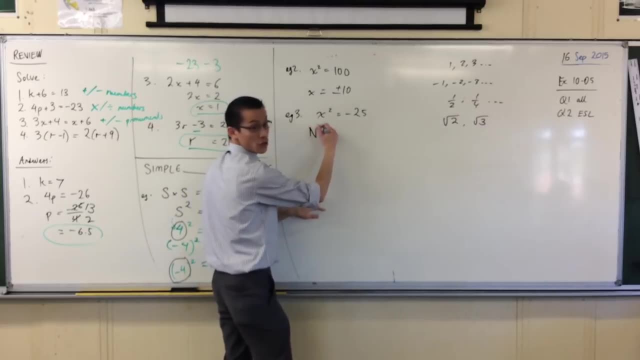 this right. None of these kinds of numbers will ever fit this kind of equation, okay, So, therefore, what I write under here, and so should you, is, I would say, no real solution. Okay, Now you might ask: well, why? why is it that I say real Like? why don't I just 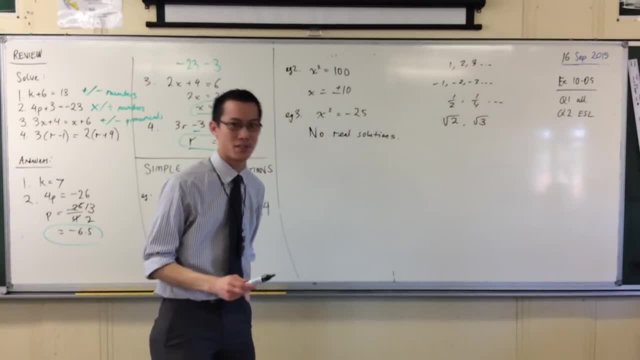 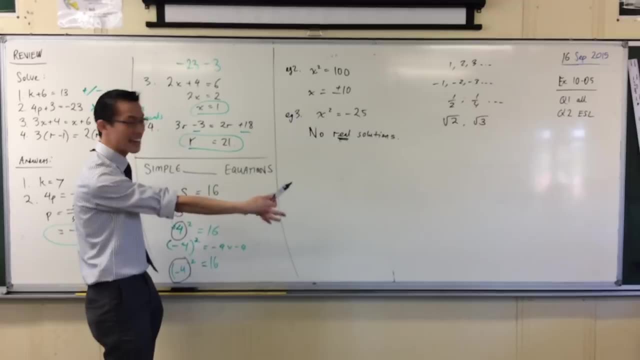 say no solutions And the answer is: there are solutions but they aren't what we call real And we will learn about those in the future. There are big, exciting, different kind of maths. just like every time you learn about a different kind of number, it lets you do new kinds of. 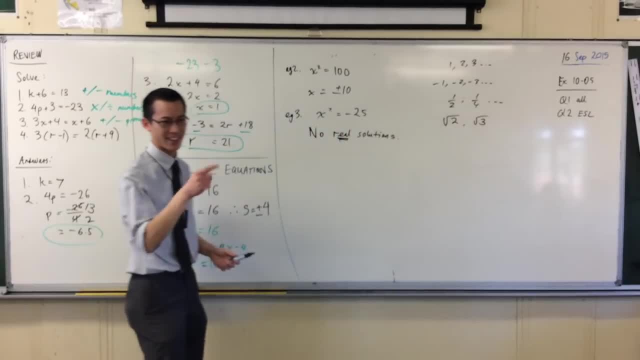 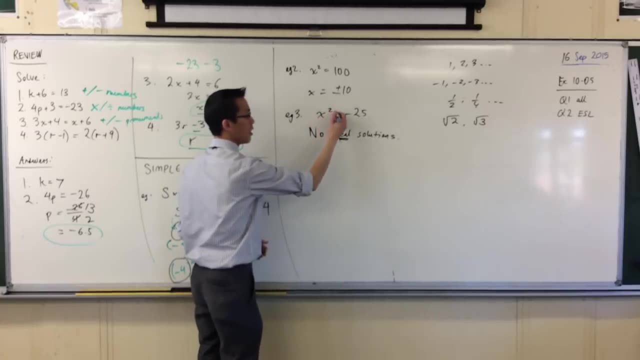 stuff, And that's the same thing with this, but that's a bit of a spoiler. Okay, Yeah, Couldn't you have one number that's negative one and it's positive, because then it's Okay, You could, but then that wouldn't be square. 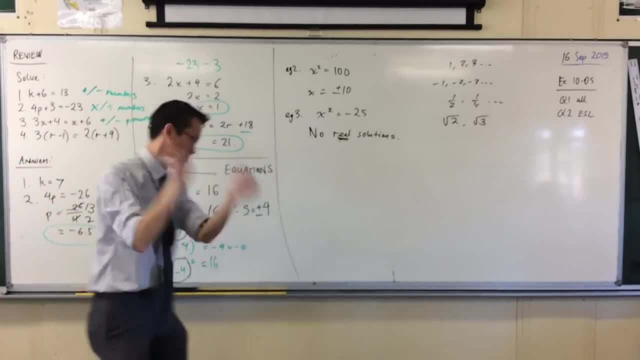 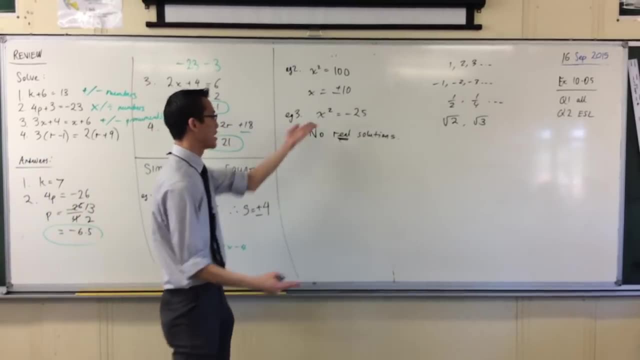 Would it? Because, by definition, square means take the same number, the same number. Maybe it's four, or maybe it's negative four or maybe it's ten, but you've got to do the same number twice, So otherwise it wouldn't be square.